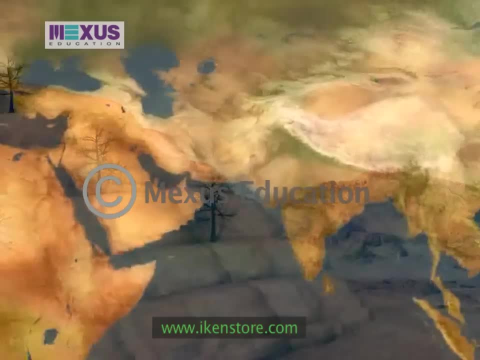 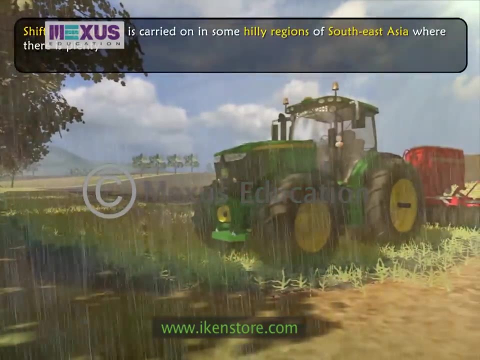 which leads to deforestation. Shifting agriculture is the oldest type of agriculture. Shifting agriculture is the oldest type of agriculture. Shifting agriculture is carried on in some hilly regions of Southeast Asia where there is plenty of rainfall and the hills are covered with thick forests. 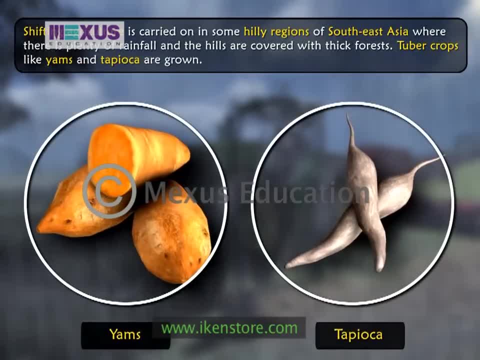 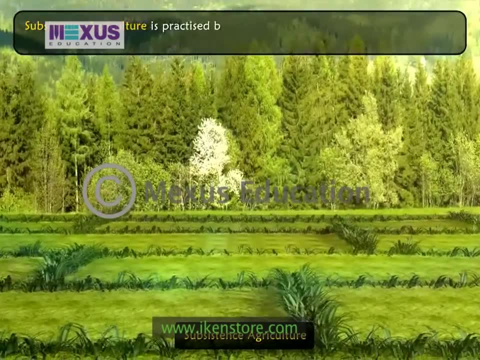 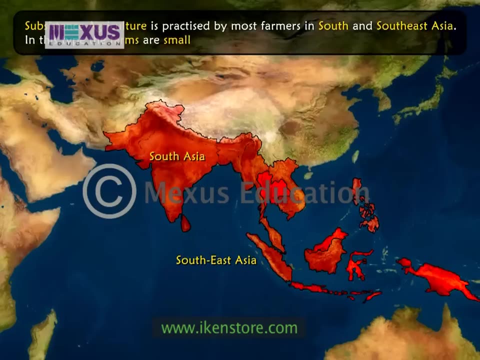 Tuber crops like yams and tapioca are grown. The second type of agriculture, subsistence agriculture, is practiced by most farmers in South and Southeast Asia. In this type, the farms are small and traditional methods of farming are followed. In this type, the farms are small and traditional methods of farming are followed. 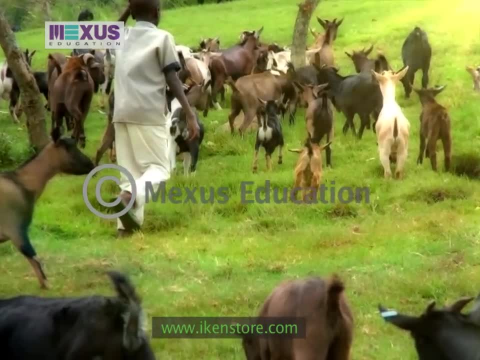 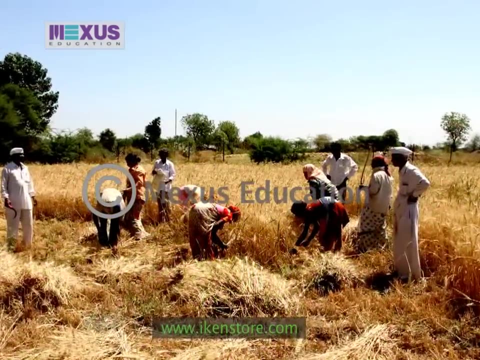 In this type. the farms are small and traditional methods of farming are followed. Much of Asia lies in the tropics and warm temperate latitudes, Hence two crops can be harvested in a year. The farmers often raise some livestock, chiefly to help with the work. 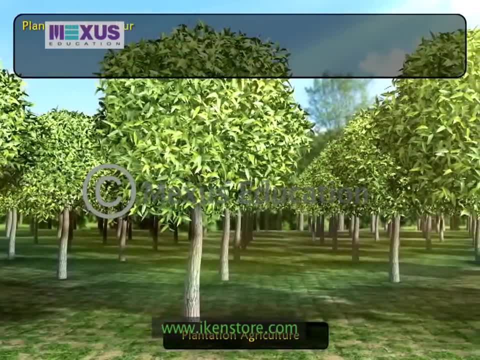 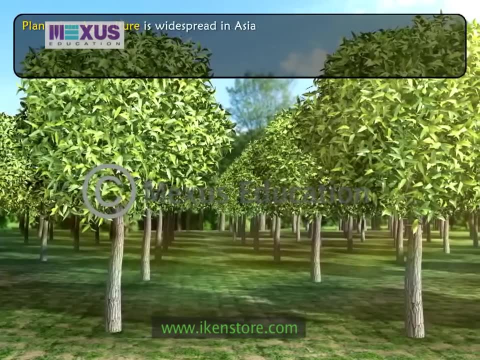 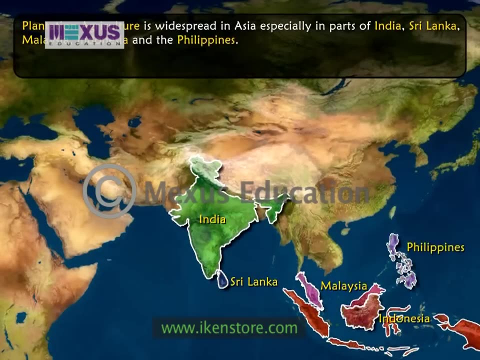 The third type of agriculture is plantation agriculture. Begun by European colonial rulers, it is also widespread in Asia, especially in parts of Asia: India, Sri Lanka, Malaysia, Indonesia and the Philippines. Here, huge estates of land are planted with a single crop. 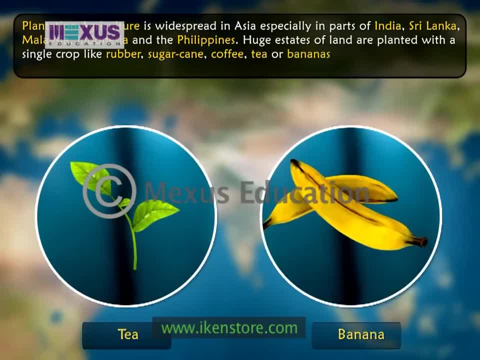 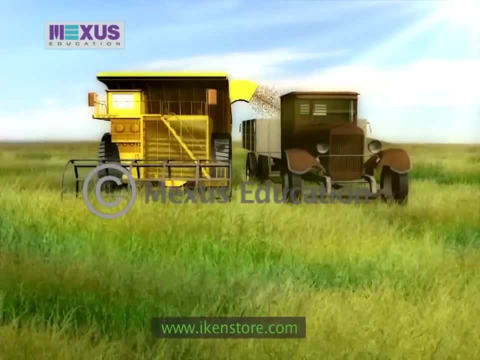 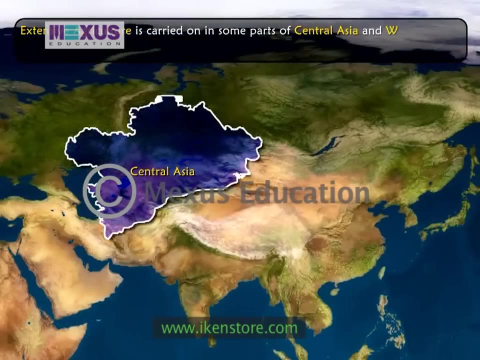 like rubber, sugarcane, coffee, tea or bananas, which are major items of export. The fourth type of agriculture is extensive agriculture, which is carried on in some parts of Central Asia and West Siberia, which is carried on in some parts of Central Asia and West Siberia. 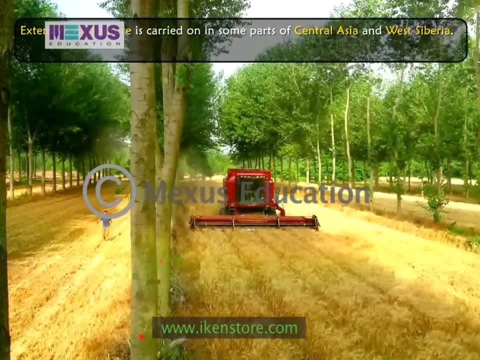 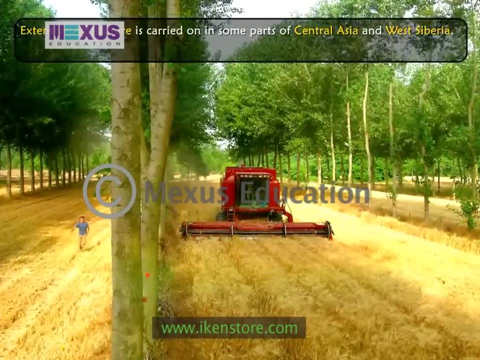 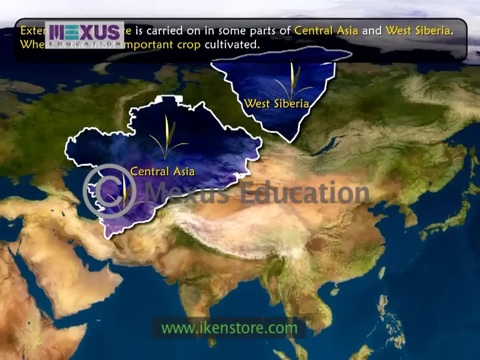 which is carried on in some parts of Central Asia and West Siberia. Due to the large size of the farm and the low density of population, manual labor is not possible. Machines are used to perform almost all farming operations. Wheat is the most important crop cultivated. 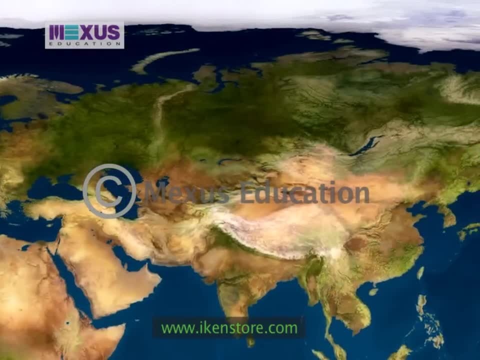 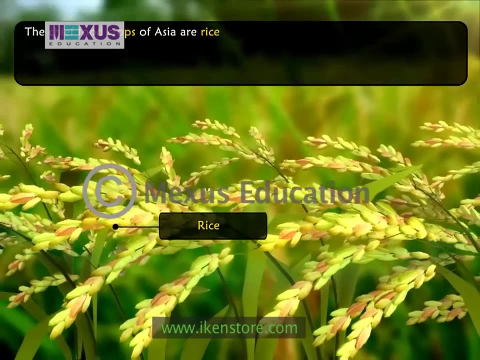 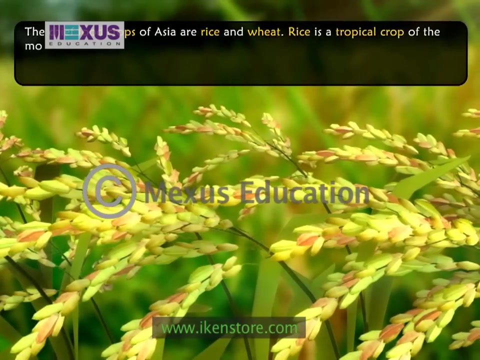 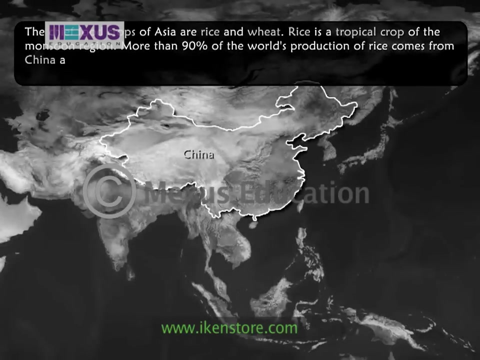 Two-thirds of the cultivated land grows food crops. The chief food crops of Asia are rice, wheat rice and wheat. wheat rice is a tropical crop of the monsoon region. more than 90% of the world production of rice comes from China and India. the other large 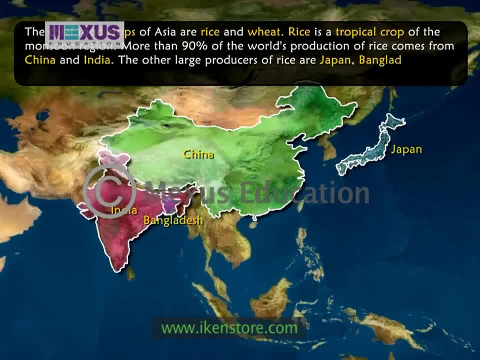 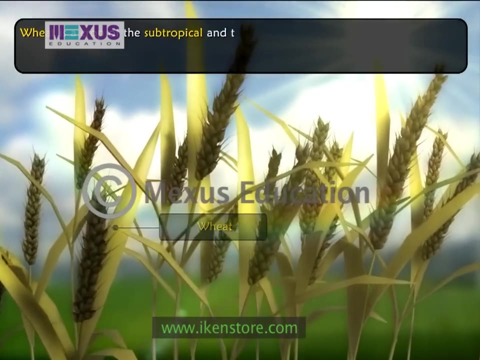 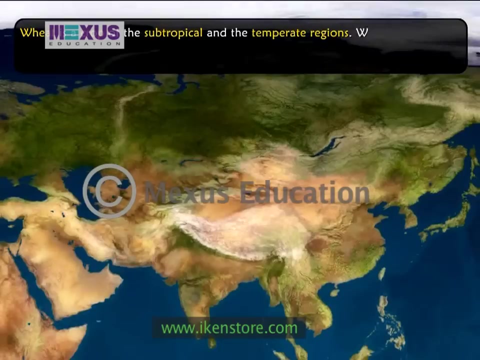 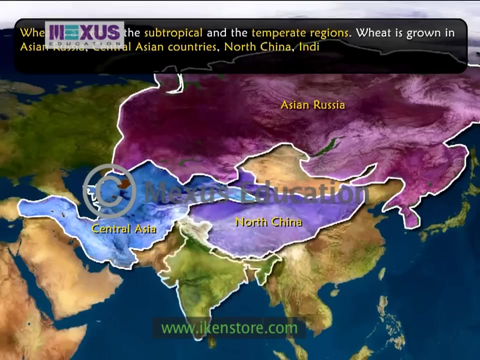 producers of rice are Japan, Bangladesh, Myanmar, Indonesia, Thailand, etc. wheat is a crop of the subtropical and the temperate regions. it grows well in cool climates with moderate rainfall. wheat is grown in Asian Russia, Central Asian countries, North China, India, Pakistan and Southwest Asia. in India and 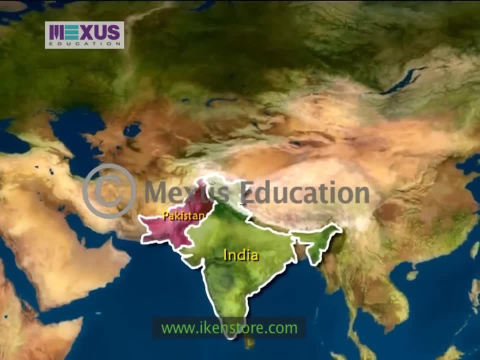 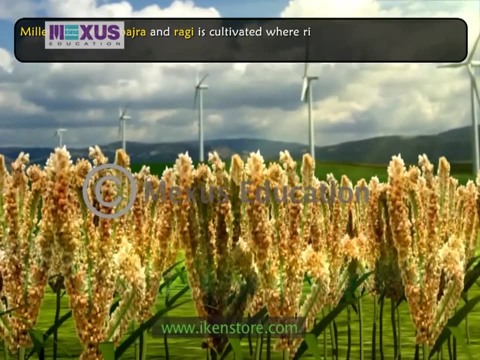 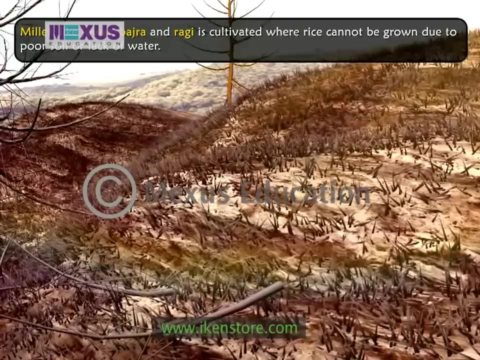 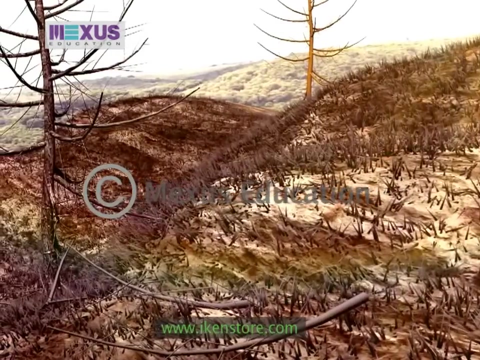 Pakistan, wheat is cultivated during the winter season. millet like Javad, bajra and ragi is cultivated where rice cannot be grown due to poor soil or lack of water. it is used as food for people and livestock. like rice, it is native of Asia and has been cultivated probably for over 7,000 years. various cash crops: 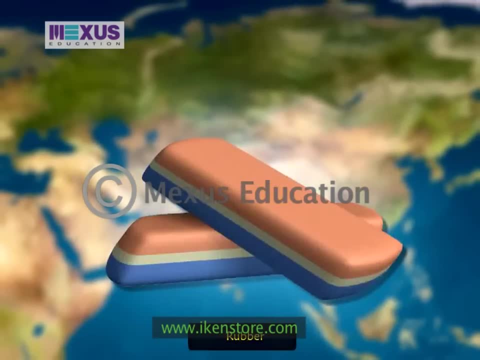 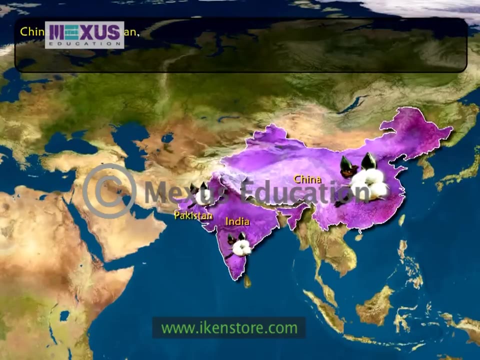 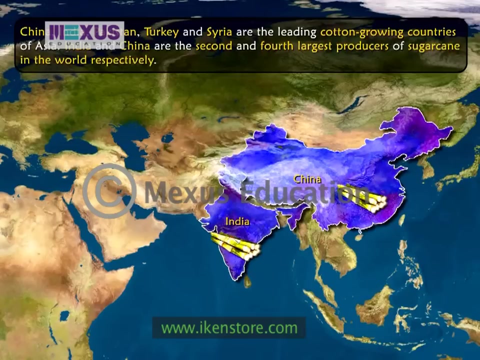 like cotton, sugarcane, tea, rubber and jute are also cultivated in Asia. China, India, Pakistan, Turkey and Syria are the leading cotton growing countries of Asia. India and China are the second and fourth largest producers of sugarcane in the world respectively. 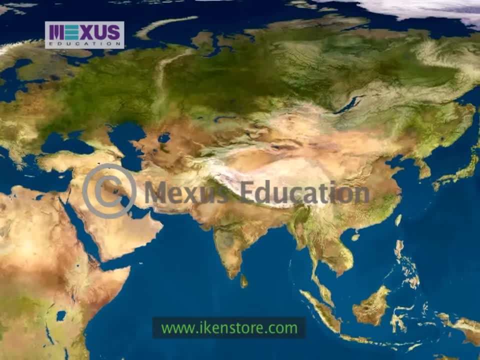 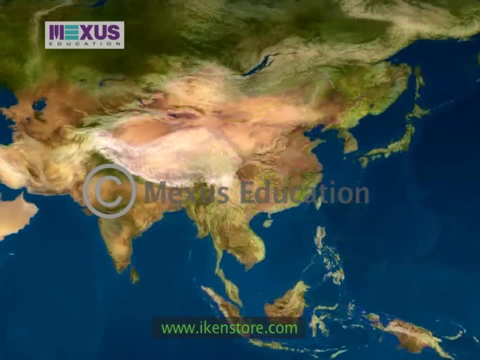 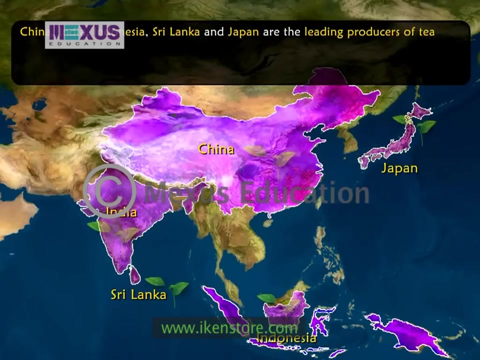 The other important producers of sugarcane are Philippines, Indonesia, Bangladesh, China and Taiwan. China, India, Indonesia, Sri Lanka and Japan are the leading producers of tea. Jute grows best in the delta of the Ganga Brahmaputra. 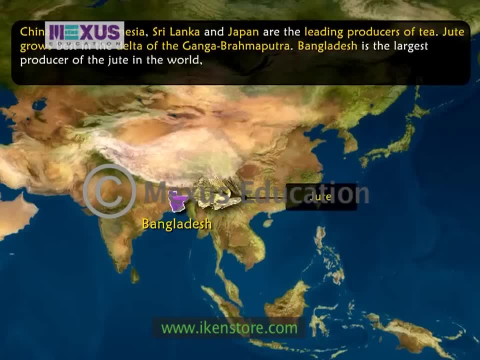 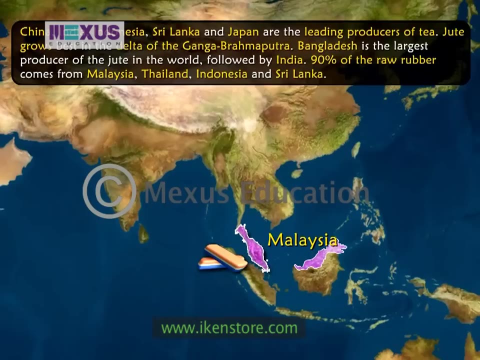 Bangladesh is the largest producer in the world, followed by India. 90% of the raw rubber comes from Malaysia, Thailand, Indonesia and Sri Lanka. Malaysia is the largest producer of sugarcane. Thailand is the largest producer and exporter of rubber in the world. 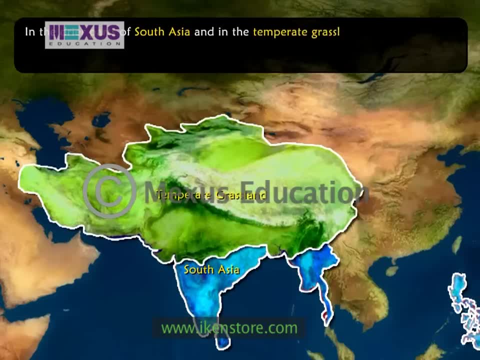 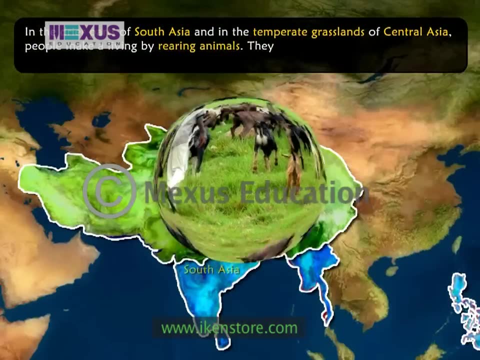 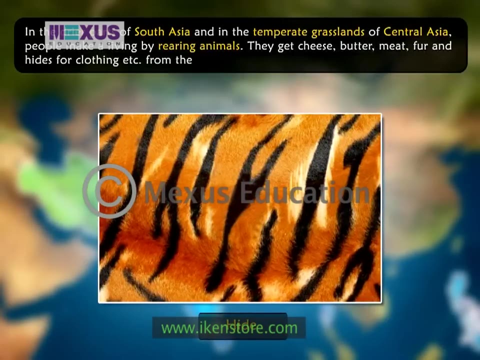 In the drier parts of South Asia and in the temperate grasslands of Central Asia, people make a living by rearing animals. They get cheese, butter, meat, fur and hides for clothing, etc. from the animals. Some animals are used for transportation. 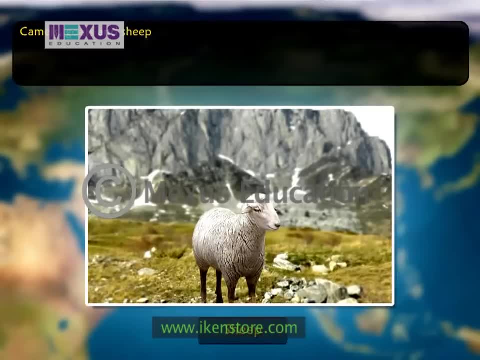 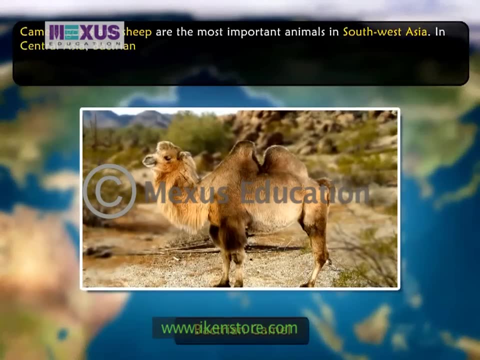 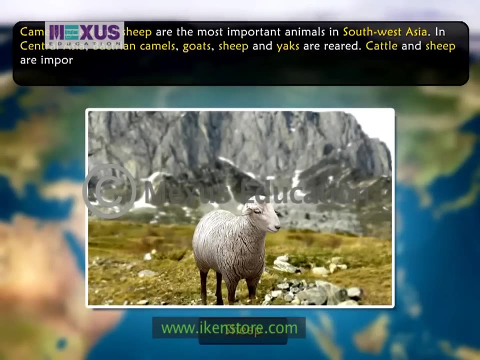 Some animals are used for transportation. Camels, goats and sheep are the most important animals in South West Asia. In Central Asia, Bactrian camels, goats, sheep and yaks are reared. Cattle and sheep are important in the temperate grasslands. 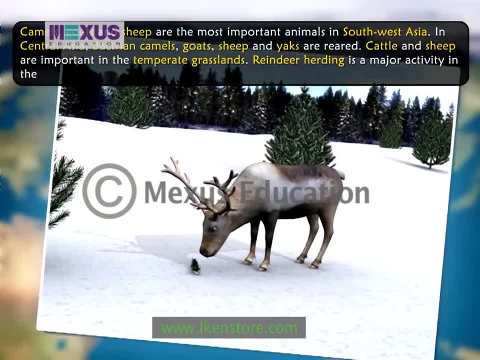 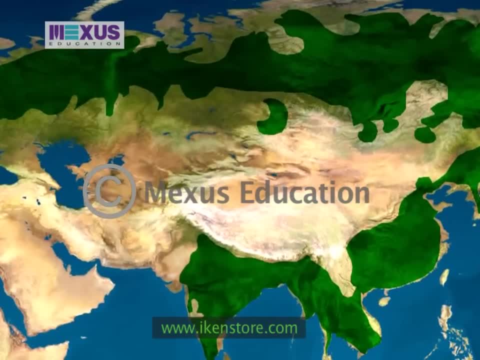 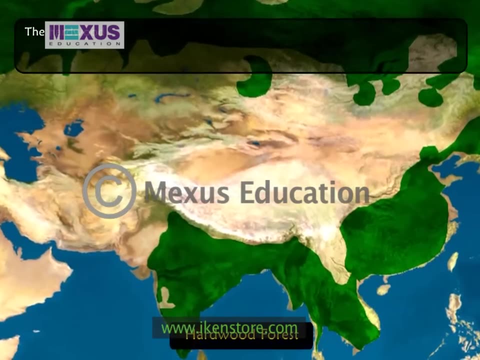 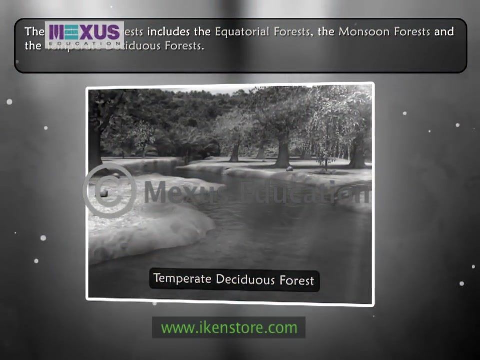 Reindeer herding is a major activity in the North Asia, has large areas covered with two main types of forests, The main types of forests which provide valuable forest products. The first type of forest is a hardwood forest, which includes the equatorial forest, the monsoon forest and the temperate deciduous forest. 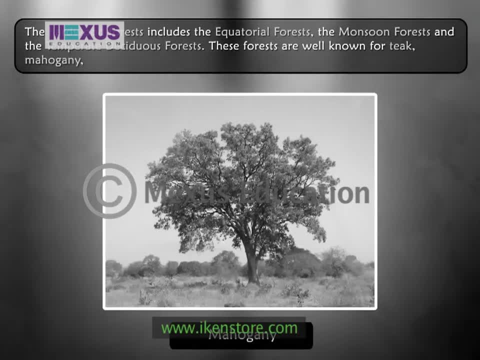 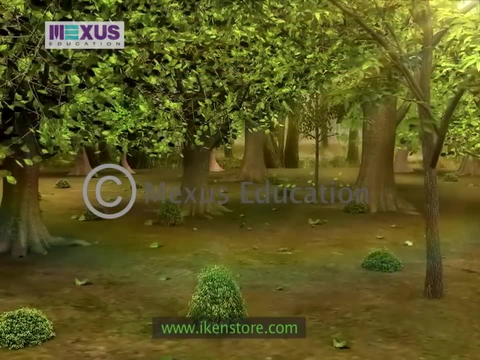 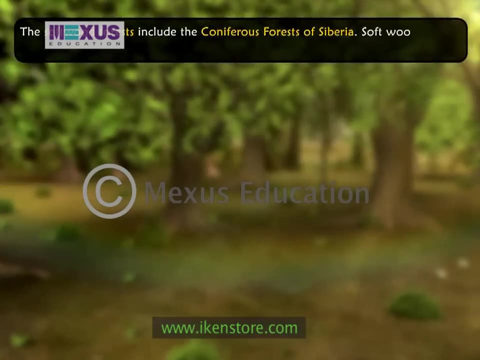 These forests are well known for teak, mahogany, rosewood, bamboo, sandalwood and camphor. The second type of forest is a softwood forest, which includes the coniferous forests. the cell soft wood is used for making paper, pulp, synthetic textiles and matchsticks. 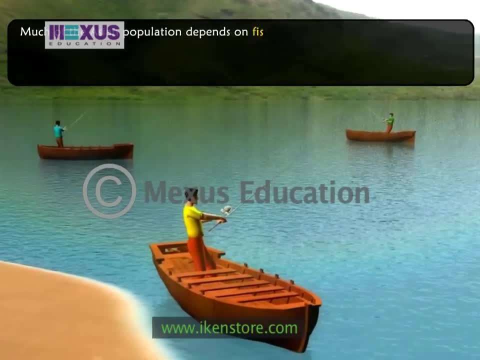 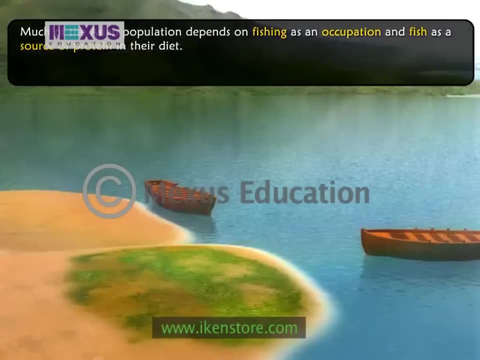 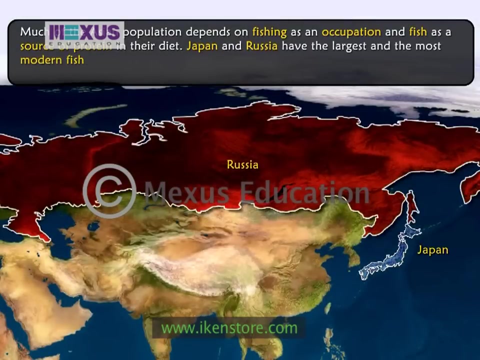 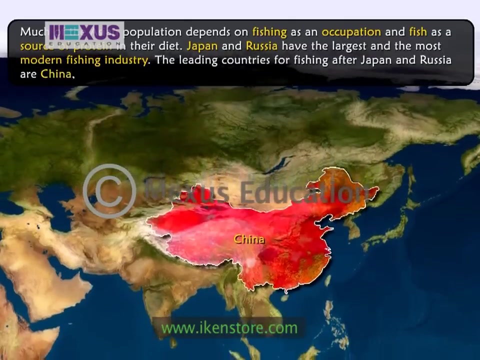 much of the Asian population depends on fishing as an occupation and fish as a source of protein in their diet. most of the fishing is done in traditional boats. Japan and Russia are the largest and the most modern fishing industry. the leading countries for fishing after Japan and Russia are China, India, Indonesia and 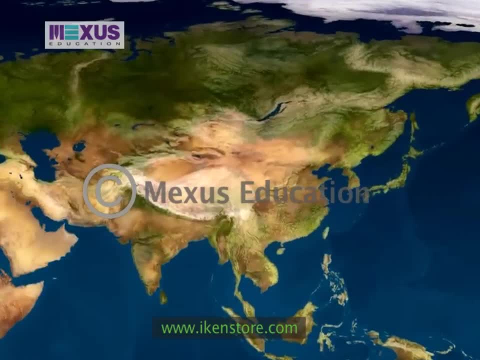 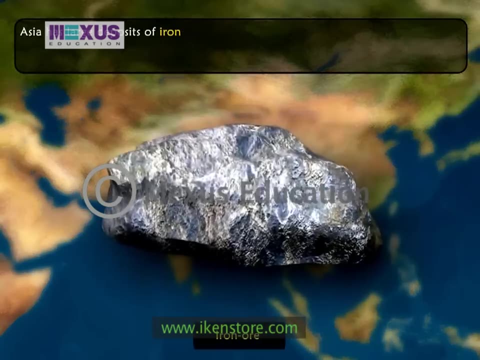 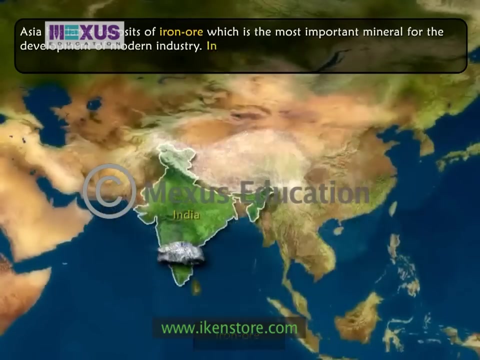 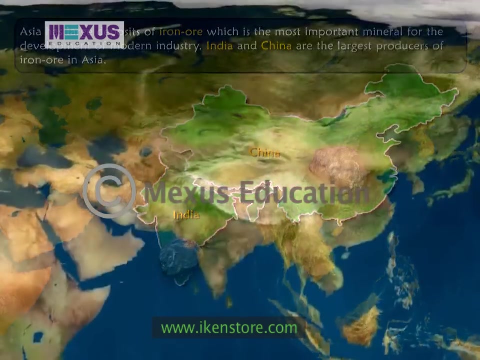 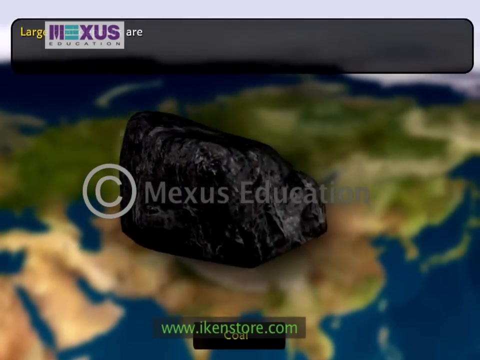 South Korea. Asia has some of the richest mineral deposits in the world. Asia has large deposits of iron ore, which is the most important mineral for the development of modern industry. India and China are the largest producers of iron ore in Asia. about 50% of coal reserves are found in Asia. large coal deposits are found in western